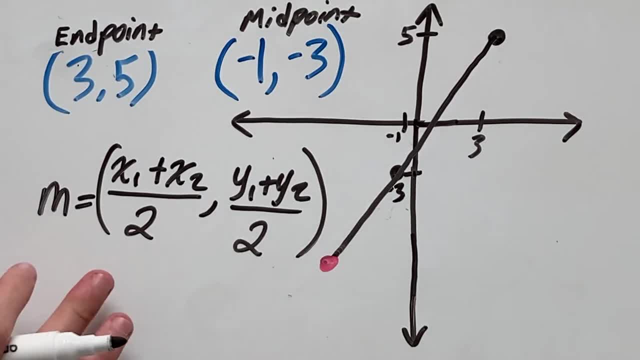 So if we rewrite this formula in sections, so break it up into X and Y, we'll get an endpoint of do x. first we can pop our values in. So we do not know what x1 is, since we are trying to find that, as that's the other endpoint. So we'll just write x1 plus. but we do know. 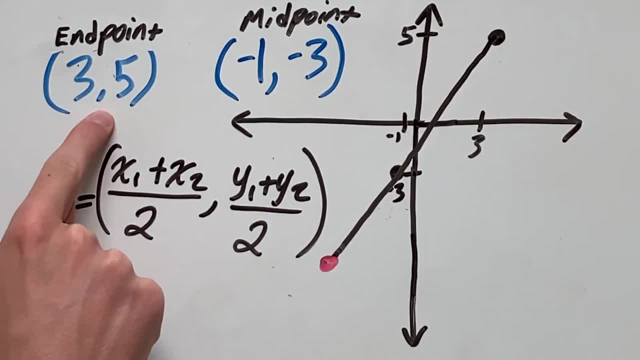 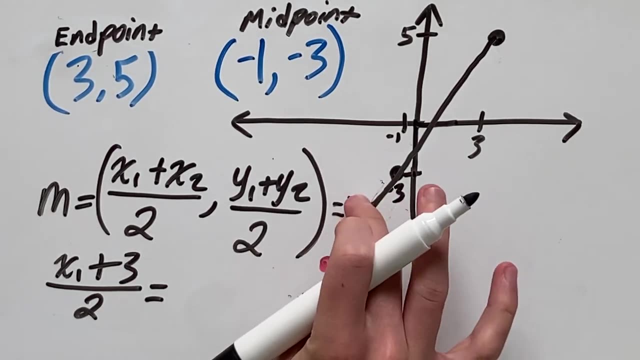 what x2 is, which is this point up here or here. So x2 is 3 over 2, and that is equal. since our midpoint is negative 1, negative 3, that is equal to negative 1,, which is the. 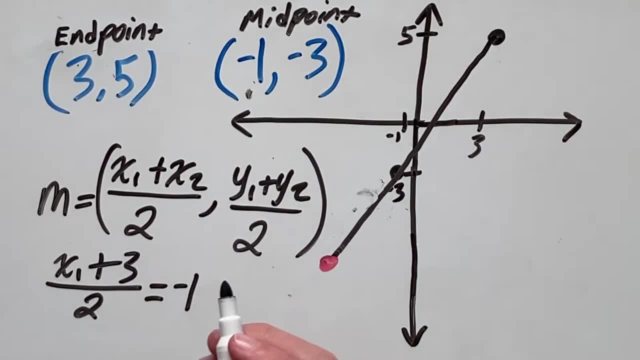 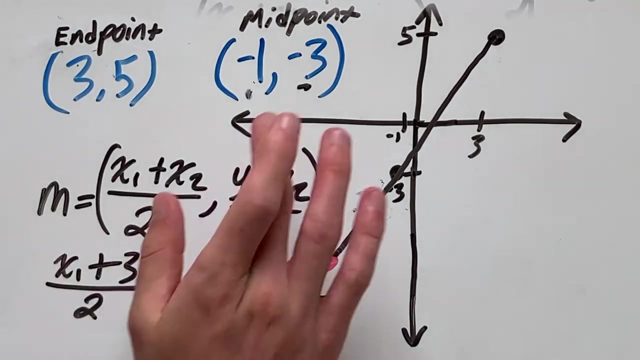 x value of our midpoint. And then we can do the same for y. So we have y1,, which is unknown since it's our endpoint, plus y2,, which is 5, over 2 equals Plus negative 3,, which is our y value of our midpoint. Now we can just focus on solving. 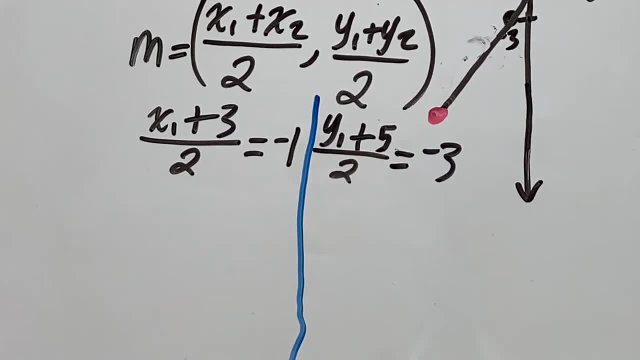 these two problems To get our endpoint. we have to solve for x1 and y1, as that will give us our coordinates for our endpoint, which we're trying to find. So just solve this equation for x1 and this one for y1.. So first we want to get rid of this. 2 on bottom. 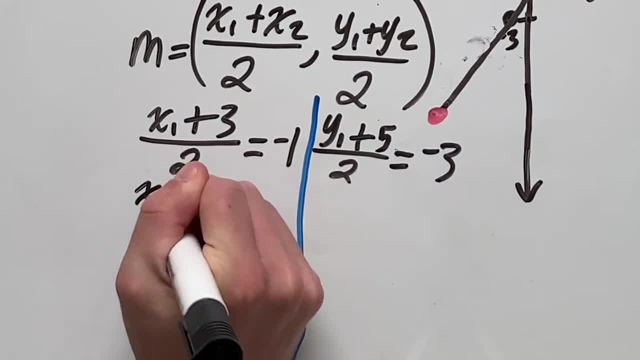 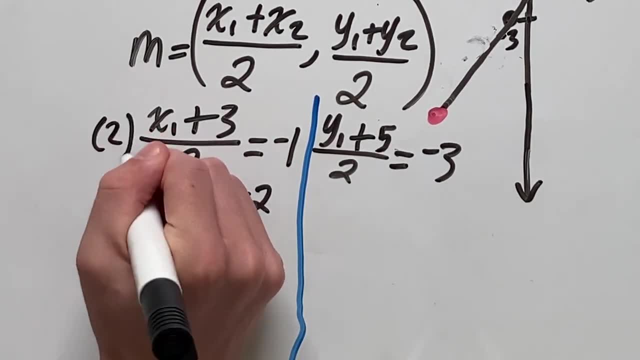 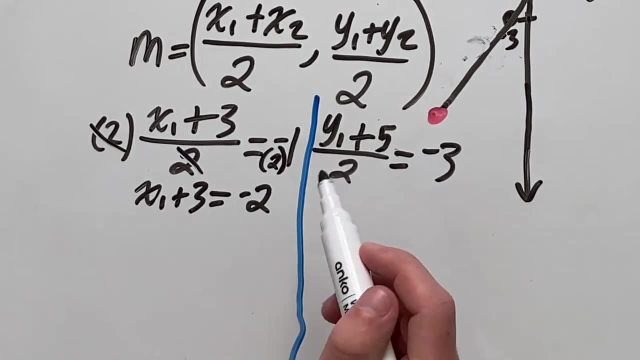 so multiply both sides by 2.. That will give you x1 plus 3 equals negative 2, since the 2 eliminated here and here, And once you multiply 2 on this side 2 times negative, 1 is negative 2.. We'll do the same on this side. Multiply both sides by 2.. That will give us y1 plus. 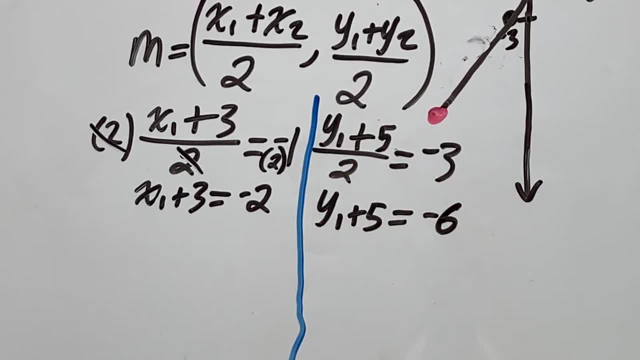 5. y1 plus 5 equals negative 6. Now we can get rid of the 3 to get x all by itself. So subtract 3 from both sides, which gives us x1 equals negative 3 minus 2, which is negative 5.. And